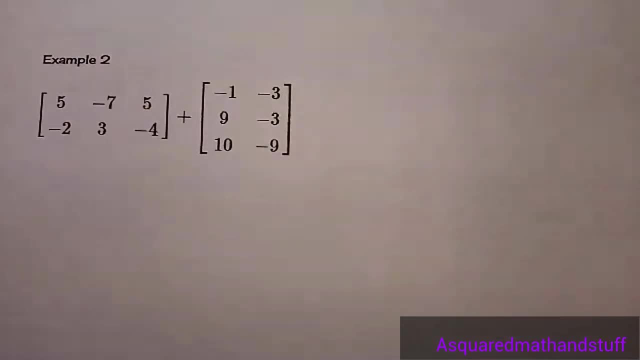 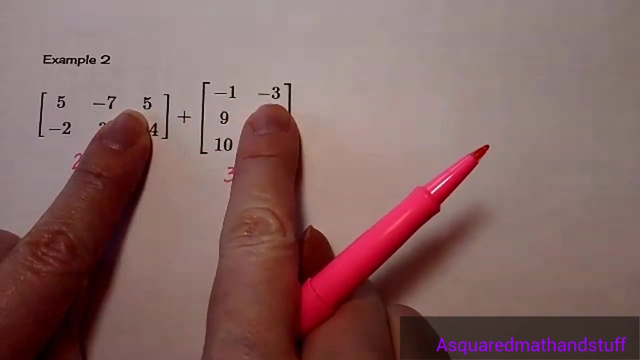 example, when we look at the dimensions, we have a 2x3 and a 3x2.. Now these dimensions are different. There's three columns in this first matrix and we're trying to be adding three columns to only two columns in the second matrix. so 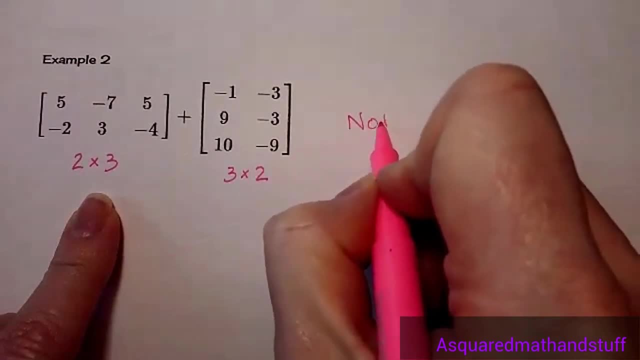 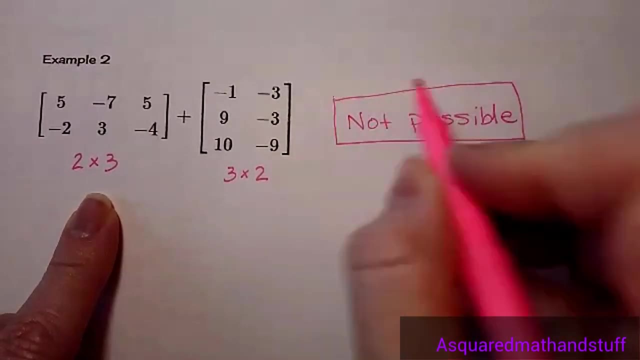 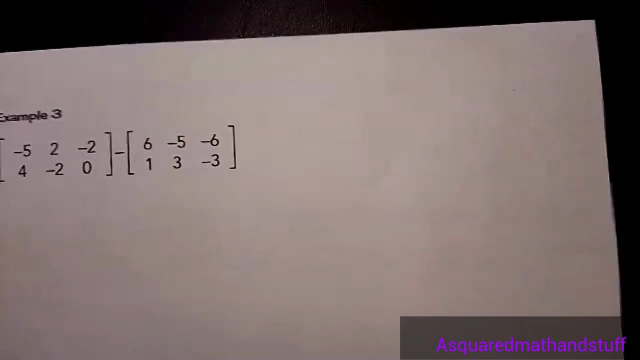 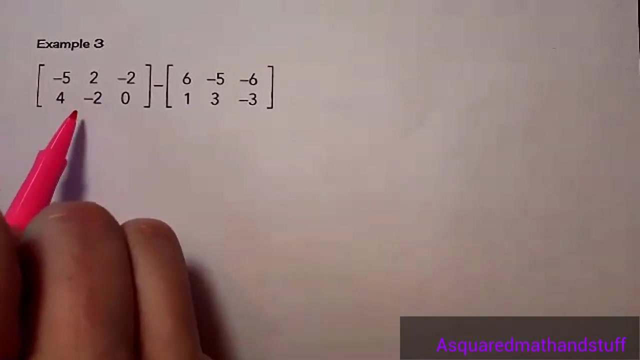 it's not possible, So we will write not possible for our answer here. The next example we will look at is subtraction. So, looking at the dimensions, we have a 2x3 subtracting a 2x3. So we are able to. 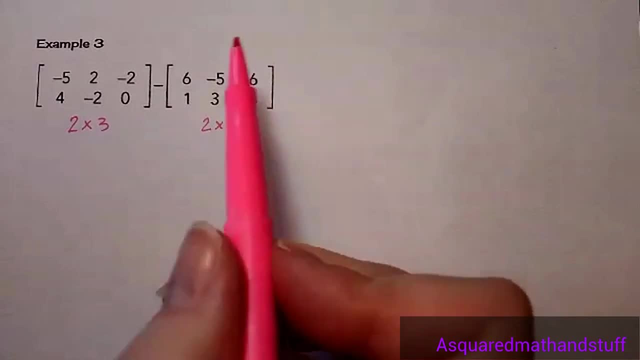 perform this operation. Don't forget: with algebra we had to distribute negative signs all the way through something in parentheses. Same process here when we're working with matrices. So this negative needs to go to every single term inside of this matrix C. Let's write that out. Row 1, column 1 is what we will work with first. 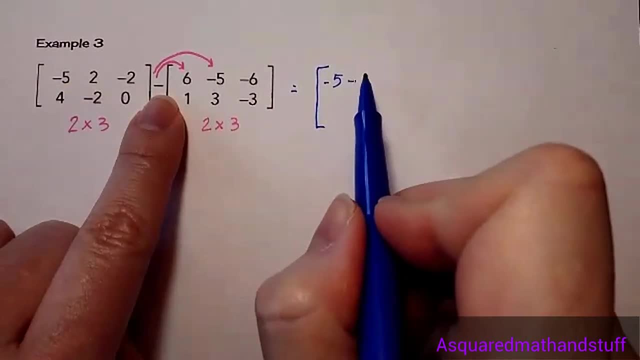 We have a negative 5 and we are subtracting a positive 6. Then we have a negative 5 and we are subtracting a positive 6. Then we have a negative 5 and we are subtracting a positive 6. Then we have a negative 5 and we are subtracting a positive 6.. 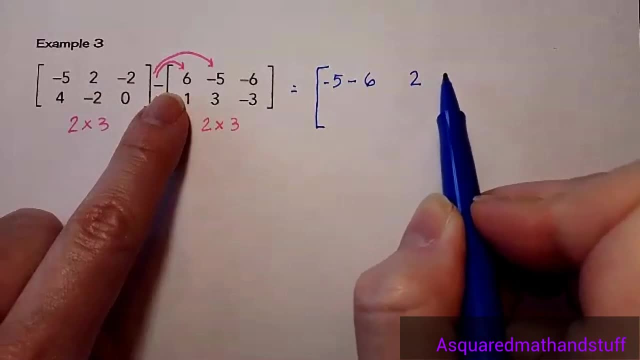 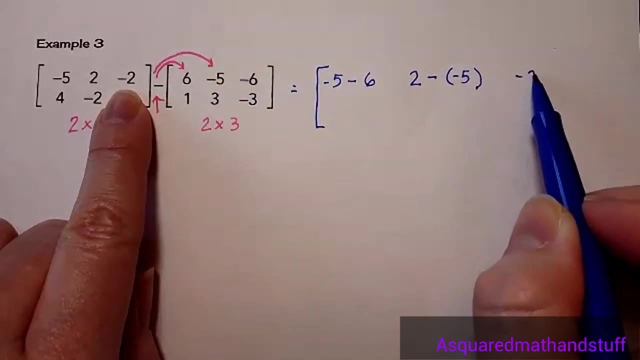 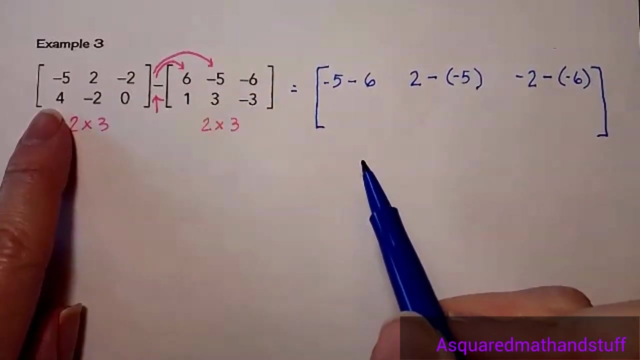 The next is row 1,, column 2.. We have a 2 and we are subtracting a negative 5.. Then row 1,, column 3.. Negative 2 minus a negative 6.. Then we do the same process, going across row 2.. So 4 minus 1.. 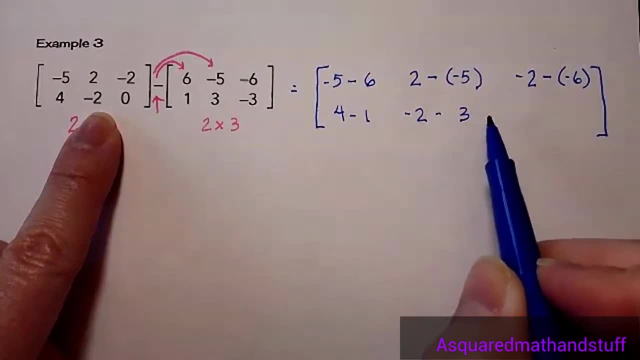 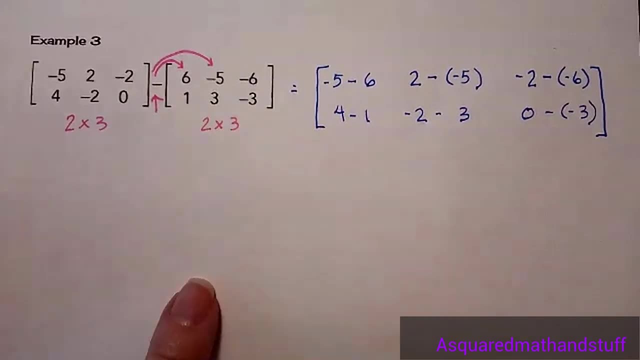 Then we have negative 2 minus 3. Then finally we have our 0. Then we have our 0 minus a negative 3. Distribute these negatives through and those will turn to positive, and then we can combine the like terms here when we have 2 negative. 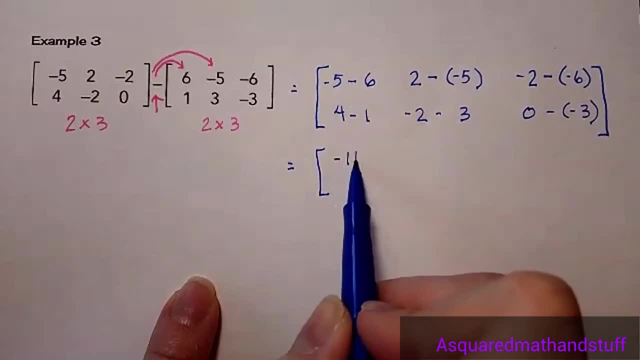 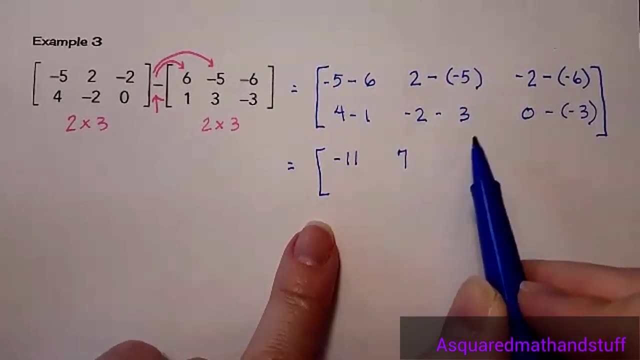 So negative 5 minus 6 gives us negative 11.. Two minus negative 5 turns this into 2 plus 5, so we get 7.. And then we have 2 minus negative 6, or negative 2 plus 6.. 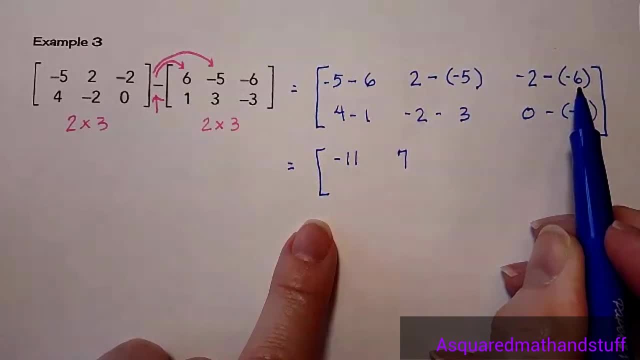 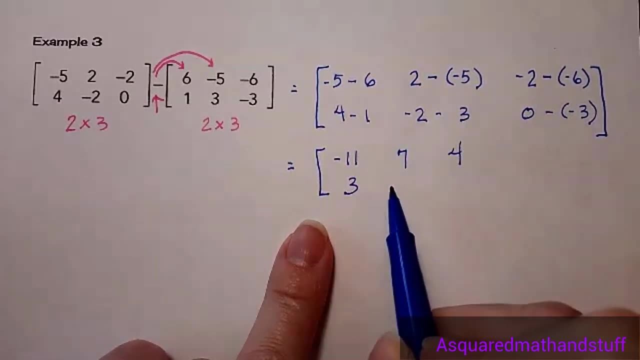 And then we have 2 minus negative 6, or negative 2 plus 6. which gives us four. Four minus one is three negative. two minus three is negative five. and then finally, zero minus a negative three gives us a positive three. 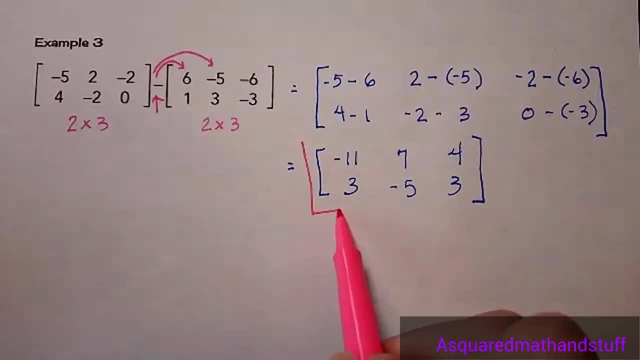 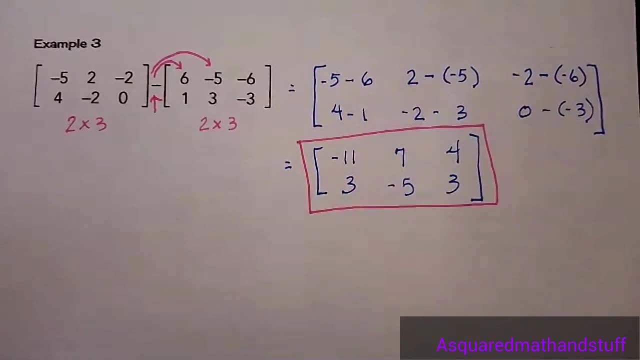 So that would be our final matrix, and that is a two by three matrix as well. so we know we did that right. for the dimensions, The last example we're going to look at combines a skill that we looked at previous to this with the addition and subtraction of our matrices. 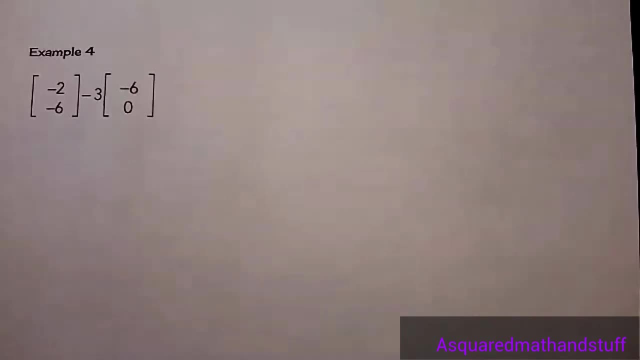 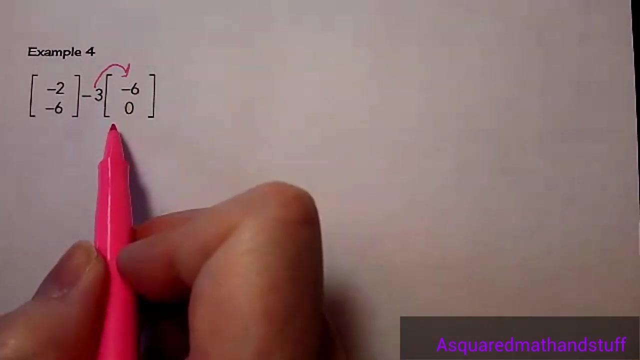 So in this one we have to look at orders of operations first. We have to multiply this three or negative three, however you want to look at it through to this matrix, And before we do that we should double check to see if we have similar operations. 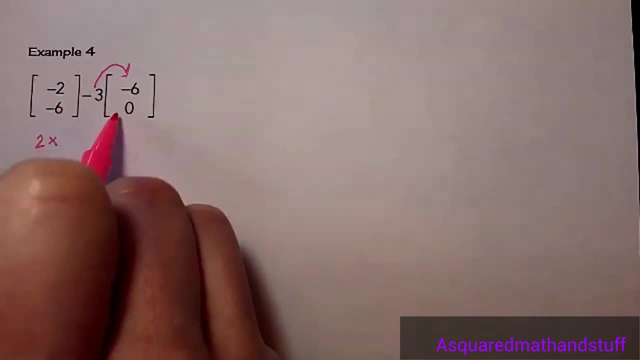 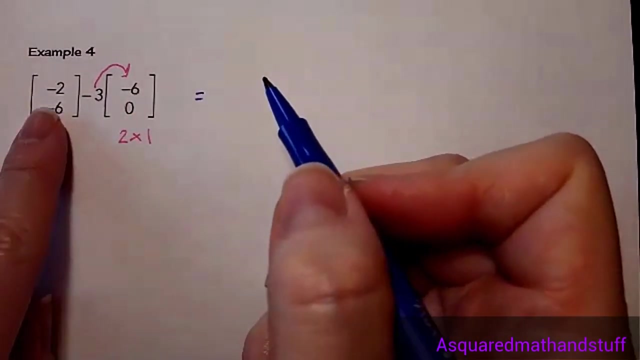 So we have a two by one, subtracting it from a two by one. So we can do this. but again, the first thing we want to do is multiply this negative three through This, then this first matrix stays the same. so we have negative two minus six. 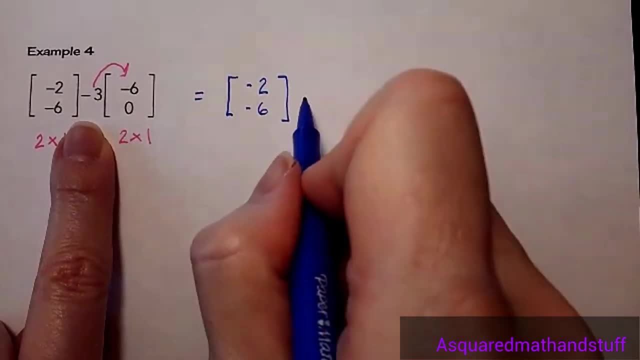 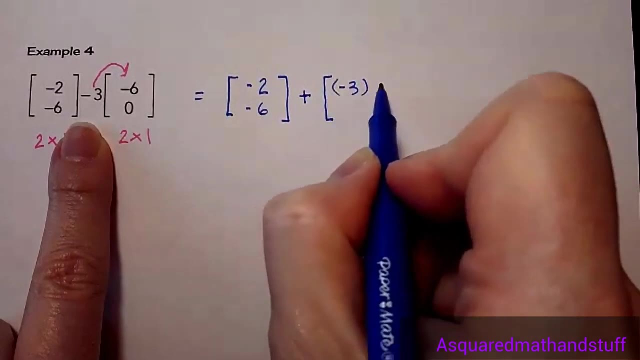 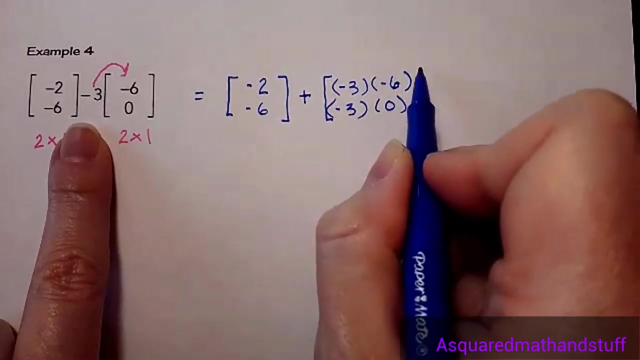 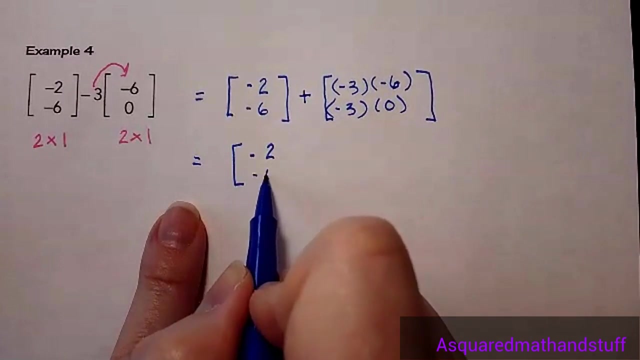 I'm going to distribute a negative three through, so I end up then. I end up then with a plus and I'll have negative three times my negative six and then negative three times zero, which then gives us the first matrix stays the same again: negative two, negative six. 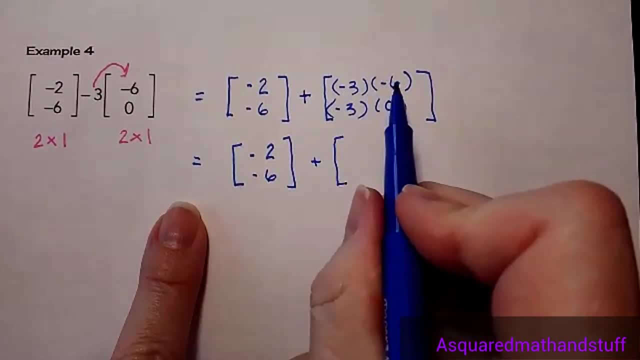 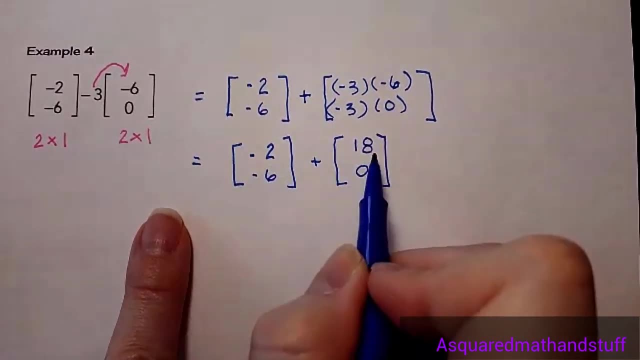 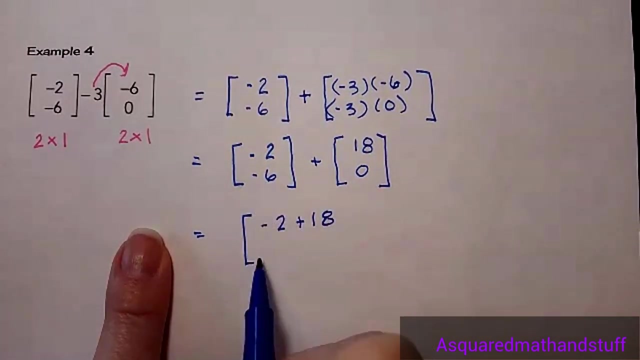 plus the matrix C of negative three times negative six is 18, and then negative three times zero is zero. Add those like positions and we end up with negative two plus 18, and negative six plus zero, for a final answer of 16, negative six. 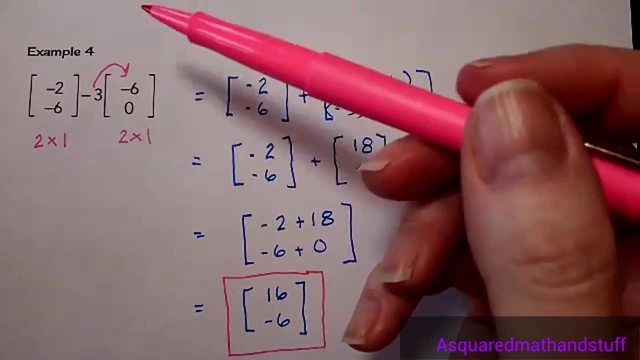 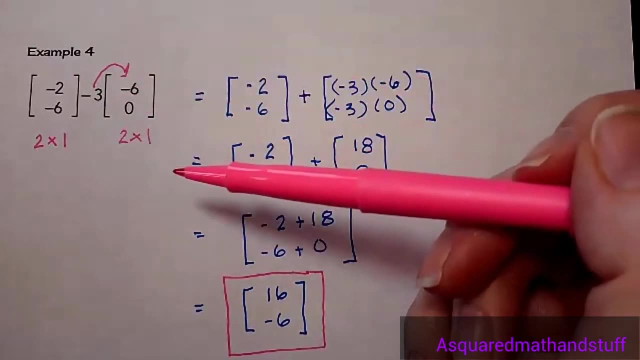 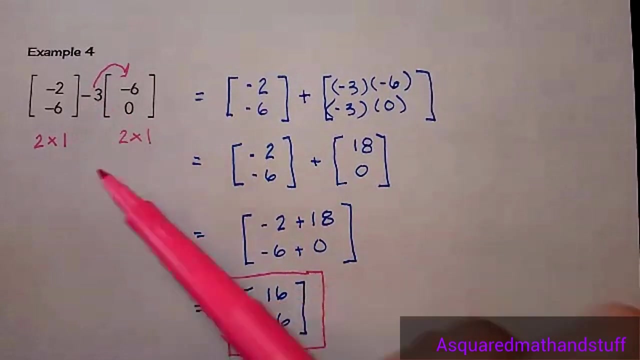 When you are given multiple matrices and different things going on, you still have to follow the order of operations that we've learned in the past, that you've applied to algebra. So again, we multiply the three through, because this is multiplication and multiplication comes before your addition or subtraction.